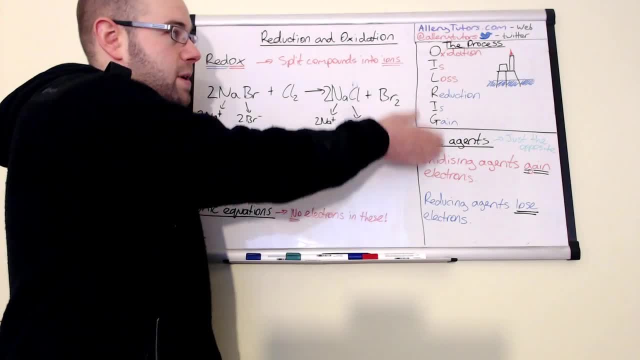 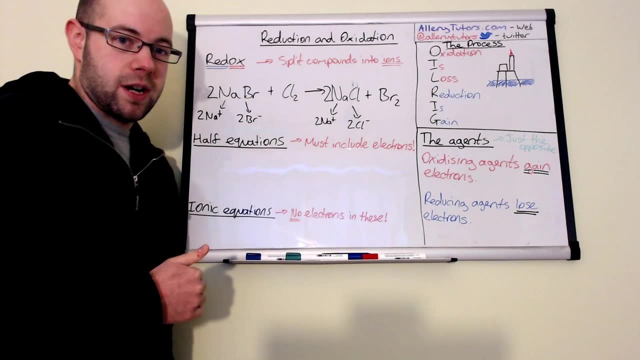 basically chemicals which do the opposite to the process, and there is a big difference between the two. So an oxidizing agent would gain electrons. So any species in a reaction which gains electrons would be classed as an oxidizing agent and any species which loses 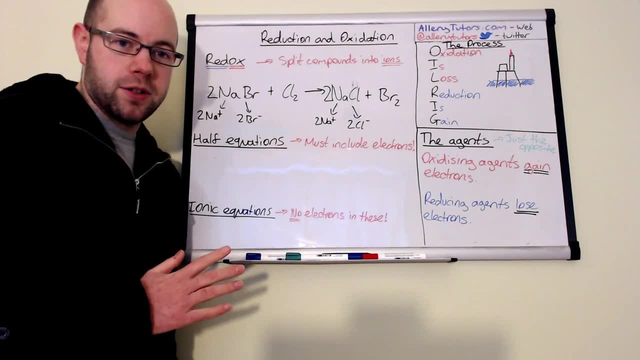 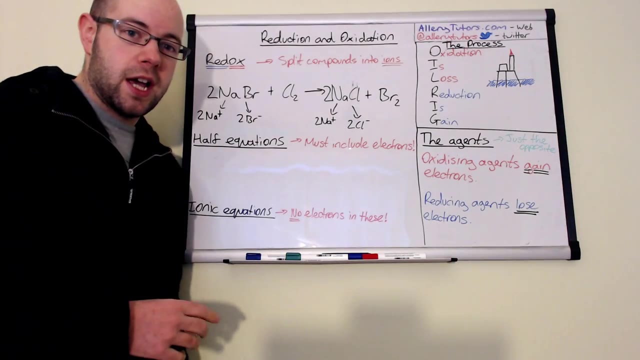 electrons would be classed as a reducing agent, and some chemicals are really good at accepting electrons, and we call them very strong oxidizing agents, and some of them are really good at losing electrons or giving up electrons, and we call them strong reducing agents. Now, actually, I'm going to use these principles here in an example and I'm going to show you. 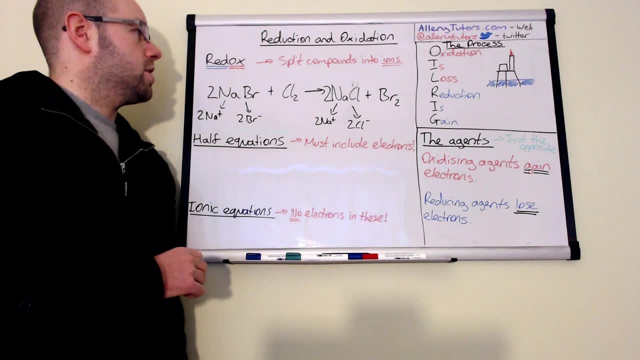 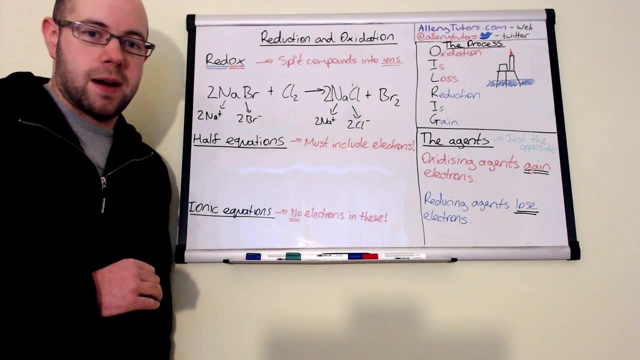 how you can write half an ionic equation. So we're going to look at this redox reaction first. Now, redox reaction is a chemical reaction that has reduction and oxidation happening at the same time, When we actually are faced with a redox equation we have to come up with. 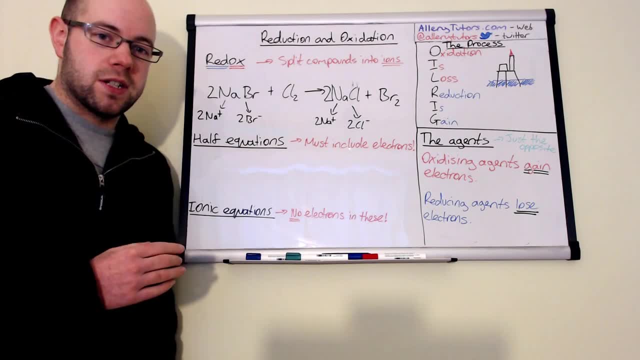 an ionic equation for this, and then the first thing we have to do is take our compounds and split them up into ions. Now, the reason why we do this is because this reaction is almost always a redox reaction. The reason why we do this is because an ionic reaction. 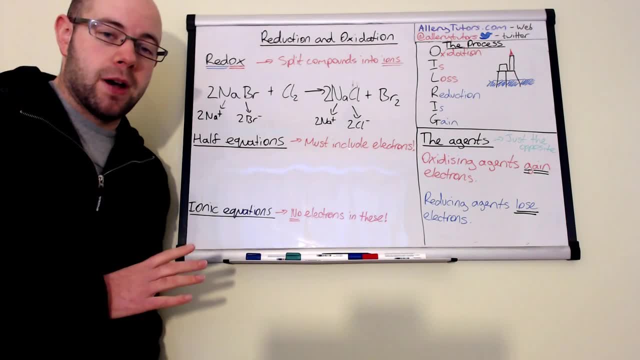 is almost always a reduction reaction, So the first thing we have to do is take our in solution. It's all aqueous, dissolved in solution, And compounds such as sodium bromide, sodium chloride, like salts, will dissolve in water, And when they do that, they actually 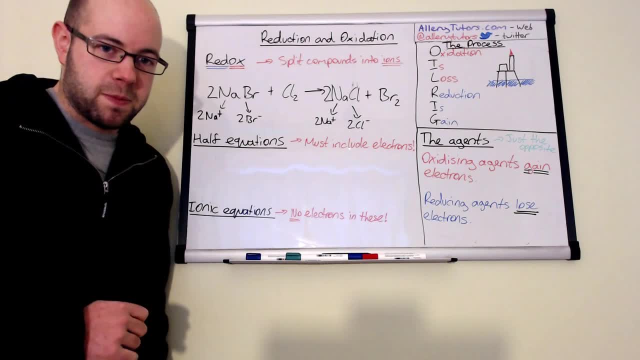 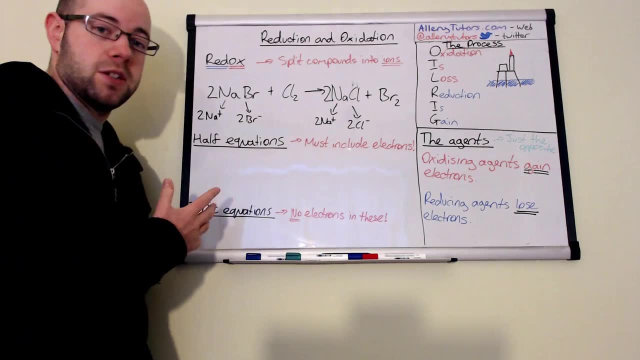 split up into ions anyway. So we're just getting a true perspective on this. So you can see, here we've got sodium bromide plus chlorine will form sodium chloride and bromine. Now this is a displacement reaction. Our compound is here and here. These are our two compounds. 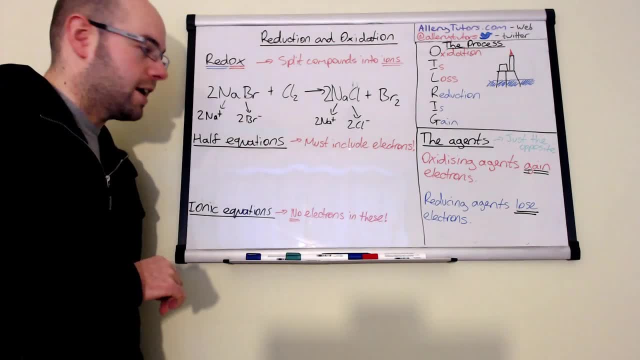 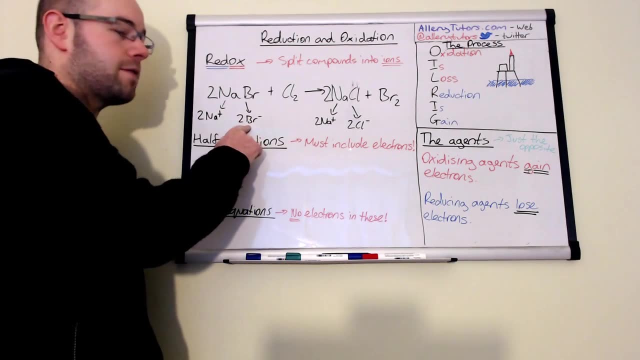 So sodium bromide will split up into the two constituent ions. So here we have two lots of Na plus, because we have two lots of NaBr. So we'll have two Na plus ions And we'll also have two Br- ions. We'll do the same over here as well, You see. 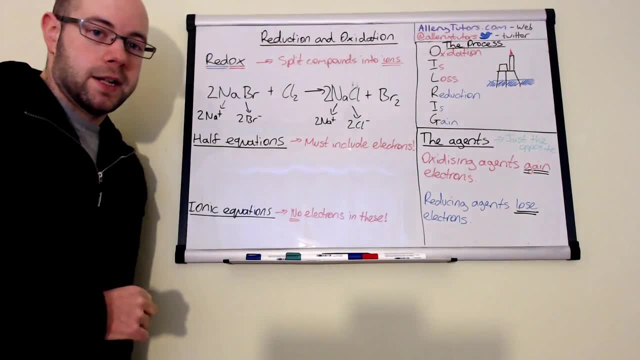 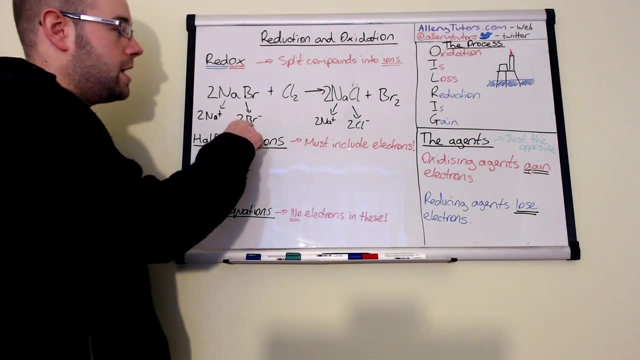 here we have two lots of sodium ions and two lots of chloride ions. Now the first thing I want to identify is basically any changes in this reaction. You can see here that the Br- has changed because it's now produced Br2.. So there's a change. 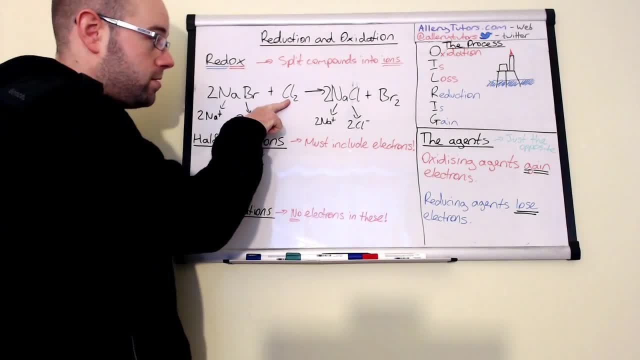 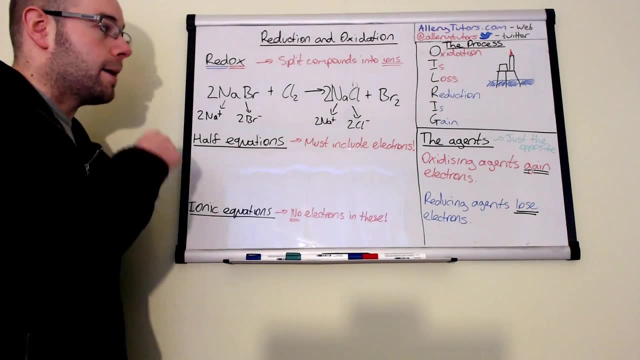 there, which I'll come on to in a minute. Our Cl2, which was a reactant here, has now gone and formed Cl- so there's a change there. Something has happened in this reaction, But you can see, the only one which hasn't changed is sodium. Now sodium has gone from 2Na+. 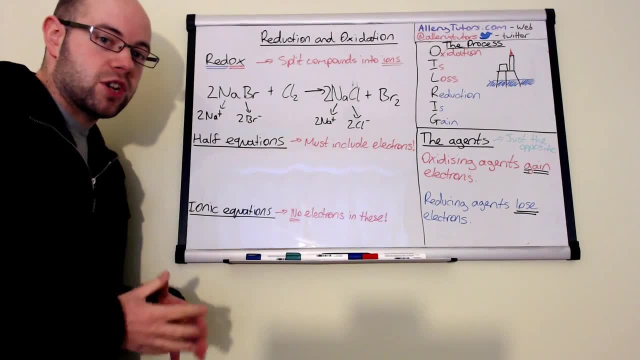 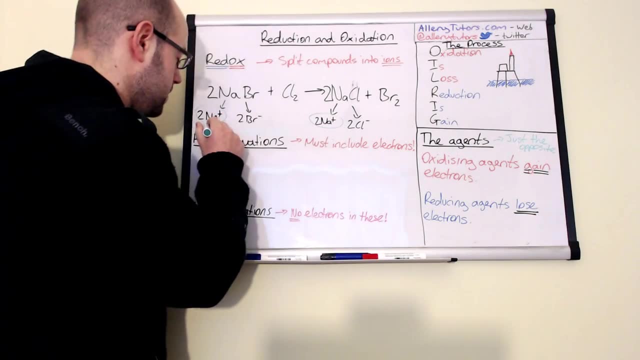 and it's still 2Na- as a product as well. So because no change has actually occurred here, we'll class sodium as a spectator ion, So I'll just circle those ones there, And these ones are spectator ions, So I'll put that one there, And so spectator ions are ions. 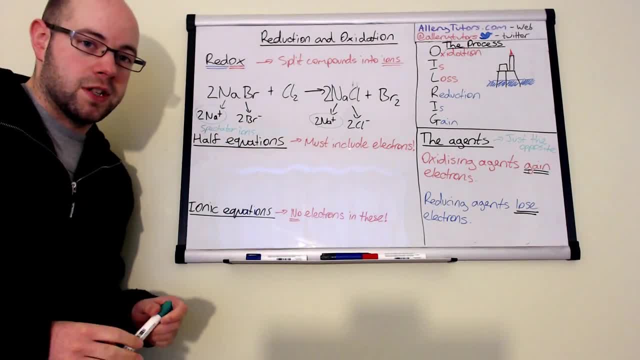 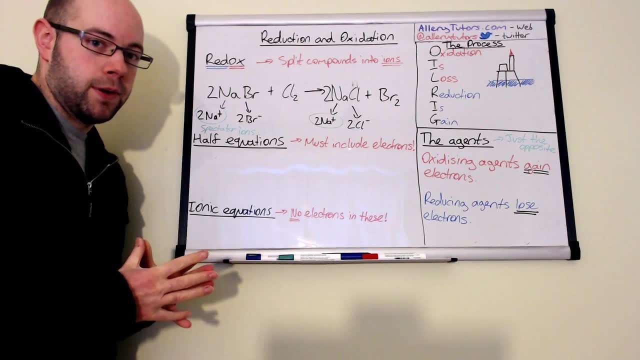 which are in the solution but they don't actually get involved in the reaction directly. So these are spectator ions there. So, looking at the ones which change, because they're the most important ones, You can see here we've got 2Br- and that's going to Br2.. We're going to write half equation. 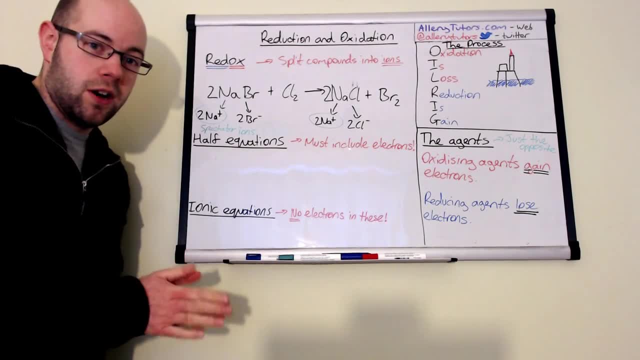 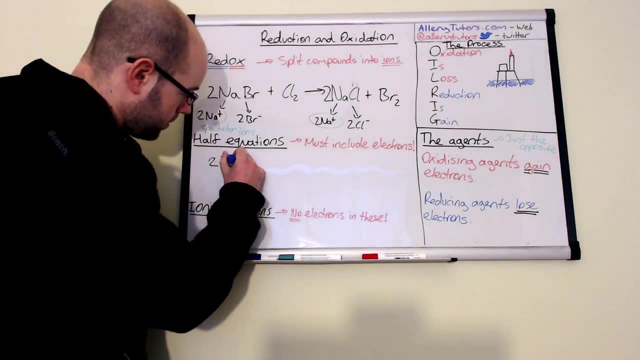 and we're going to try and identify if that is an oxidising process or a reducing process. So we're going to write half equation and we're going to try and identify if that is an oxidising process or a reducing process. So we're going to write down 2Br- because that's what we start off with. So there's our reaction. 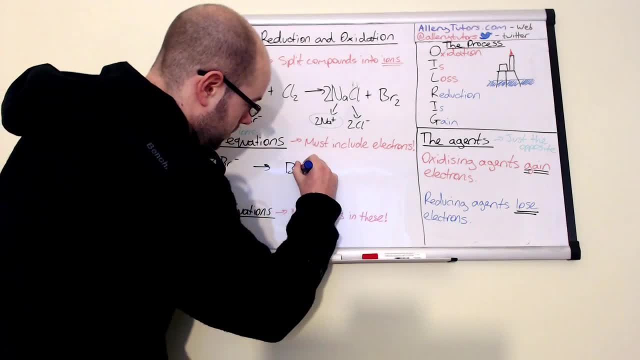 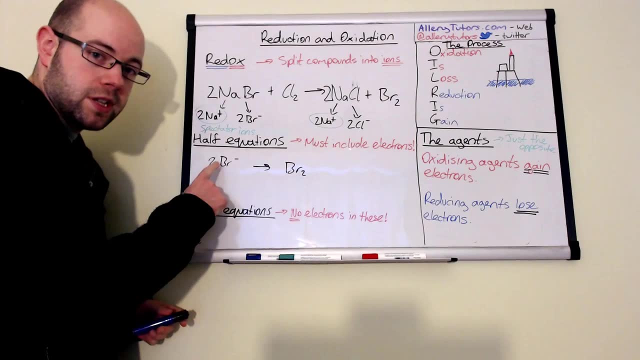 there And that's going to form Br2.. So we're going to put that there. Now you can see here that we have a 2 negative charge on here, So we've got Br- but we have two of them, so that's 2 minus. And we have Br2 over here, which is neutral. It doesn't have a charge. 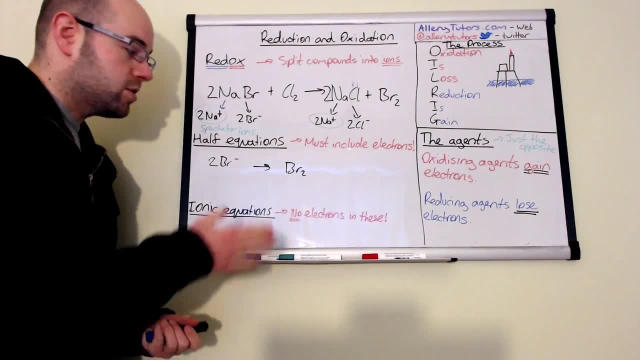 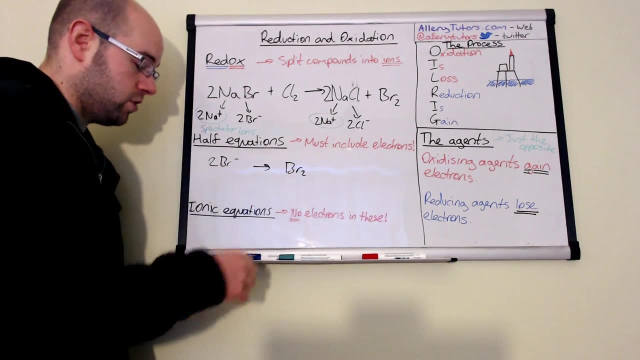 Now remember: oxidation and reduction is all to do with electrons. So we're going to add electrons here to balance out the charges on the left and the right. You can see here that obviously it's negative here and neutral here, so we need to add negative charges on this. 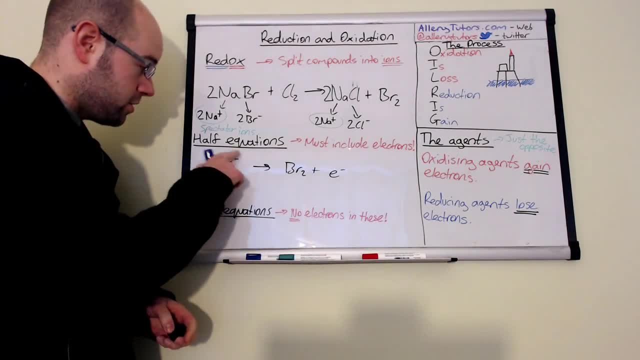 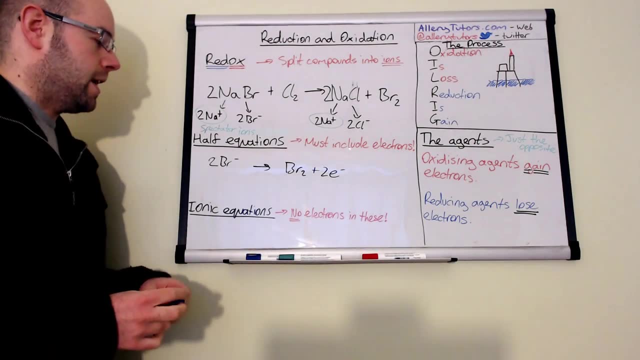 side, So we need to add an electron there And because we have a 2 negative charge there and it's neutral on this side, then we have to have 2 electrons on the right-hand side, which is on there. Okay, so try to identify if this process here is oxidation or reduction is. 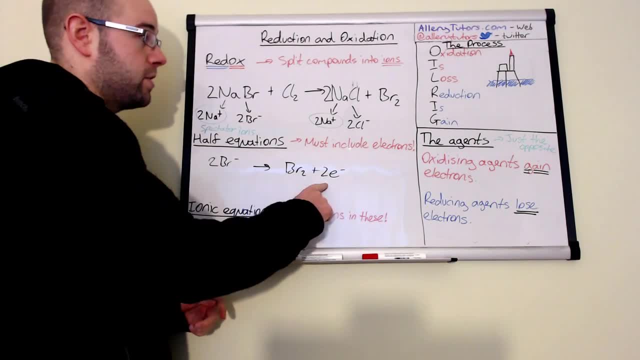 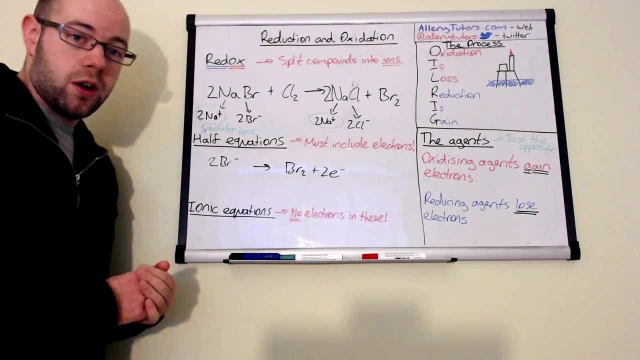 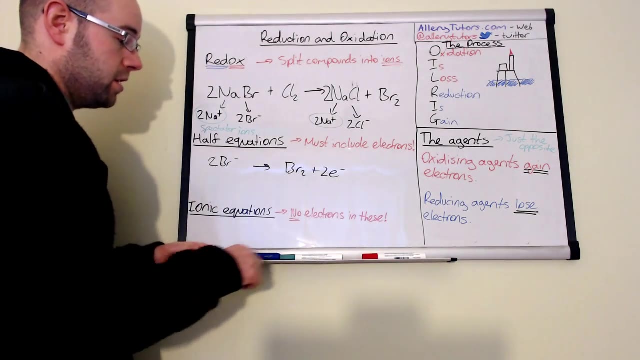 really simple. So you can see here that Br- is obviously we have a loss of electrons. so this whole process here is actually oxidation. So we're losing electrons onto obviously as we go from Br- to Br2.. So we call this oxidation. So I'm going to put that one there. 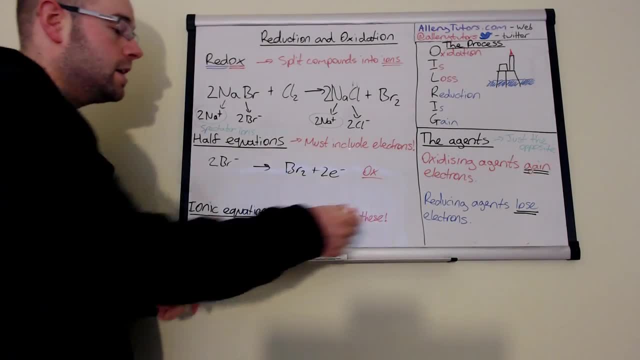 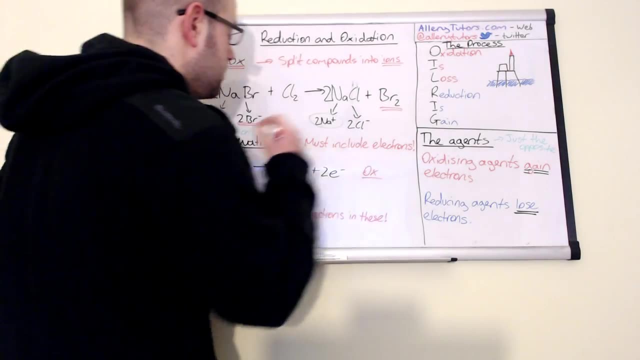 So this one's oxidation, so I'll put that one on red, Okay, so if we look at the other side, I'll just highlight this. So there's Br- go to Br2.. So this is oxidation, this process here. 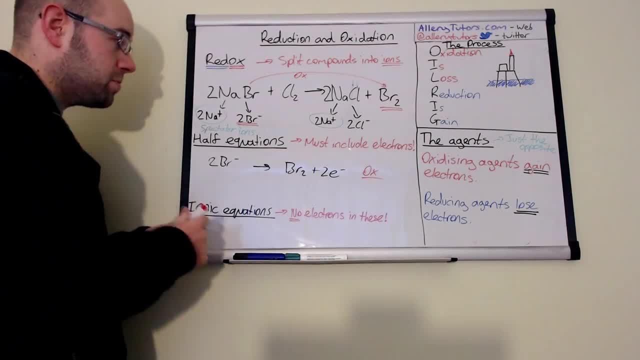 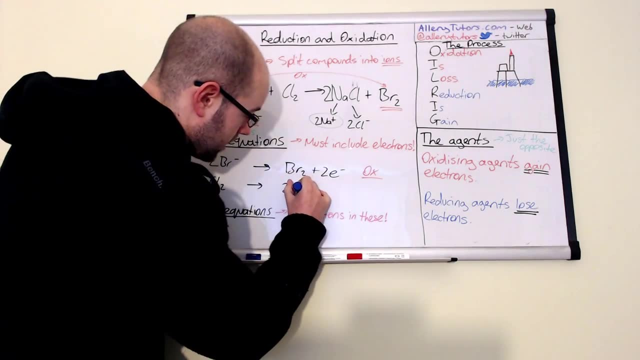 That's oxidation, Okay. the next one is Cl2, which is this one here, Cl2.. And that's going to go and form 2, lots of Cl- Now you can see that we have a 2 negative charge on the right, neutral on the left. 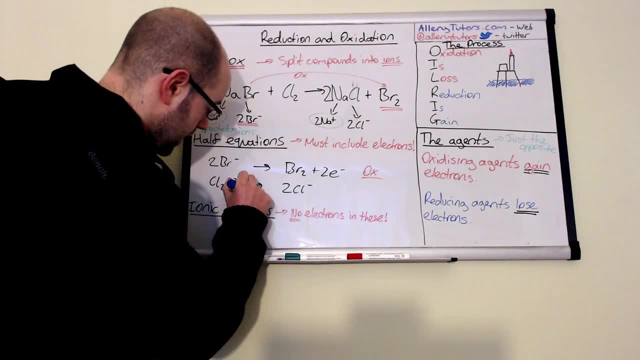 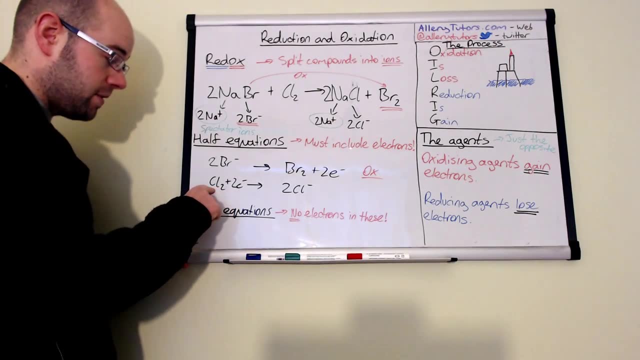 so, in terms of electrons, it has to go here: 2 electrons, 2 E- on the left-hand side. So this process, as you can see, is obviously gaining electrons. We have Cl2, accepting electrons to form Cl- So this is going to be. 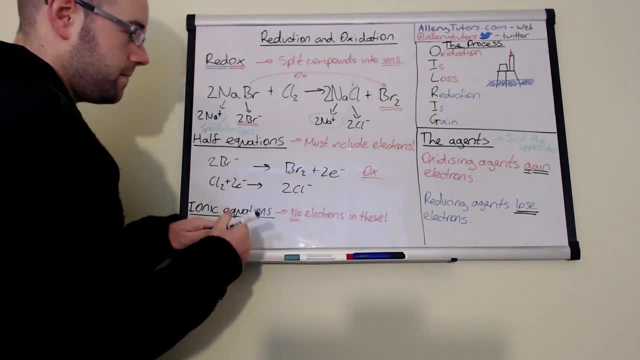 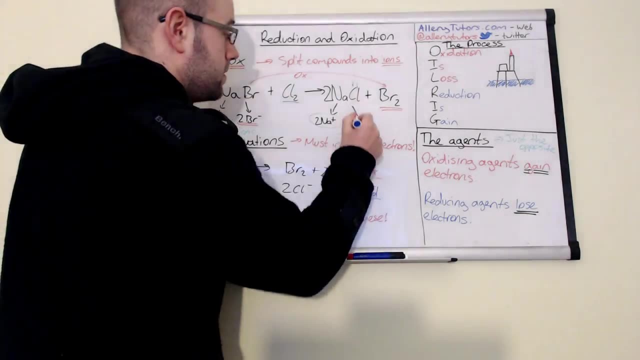 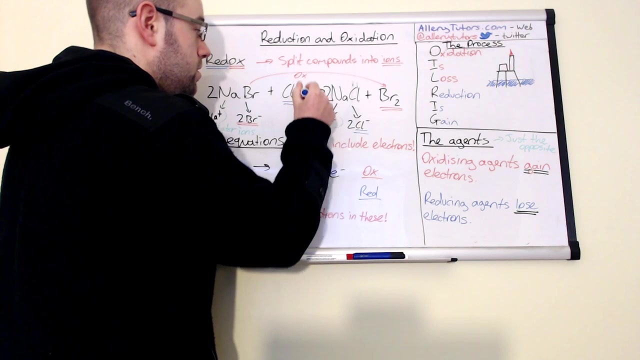 is the reduction reaction, So we're going to put this one over here. So this is reduction, So put red over there And so we'll highlight this. There's the Cl, There's the Cl- So this one is obviously going to be reduction. Going from there to there is reduction. So our chlorine. 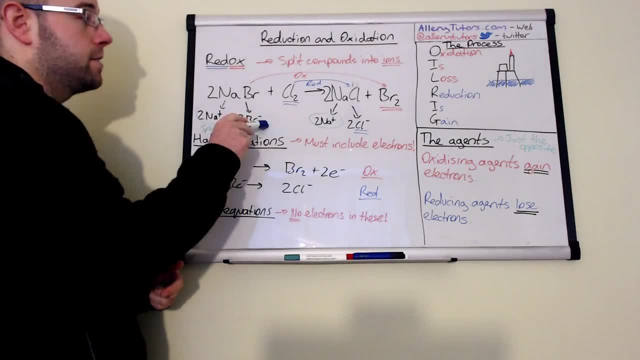 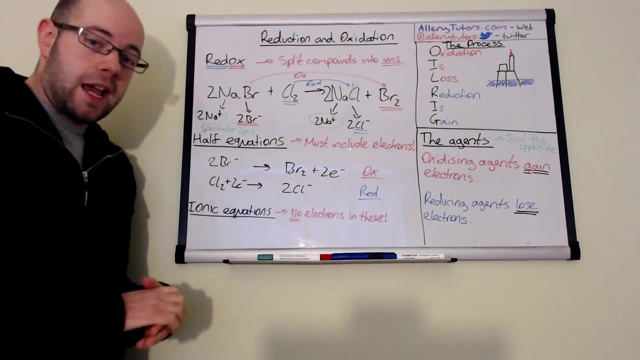 is undergoing a reduction reaction and our bromide ion is undergoing an oxidation reaction. So, in terms of the agents, remember, an oxidizing agent is something that gains electrons. If you look at these reactions here, the only one which is gaining electrons is the chlorine, So that's. 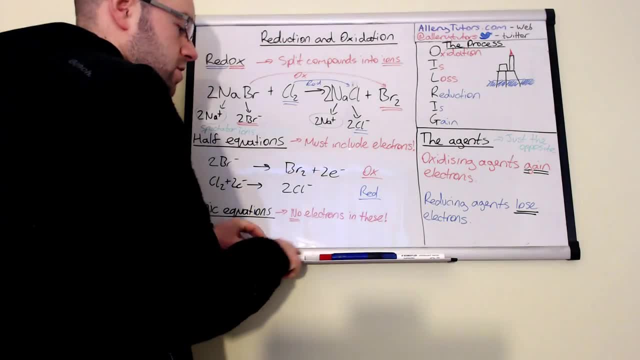 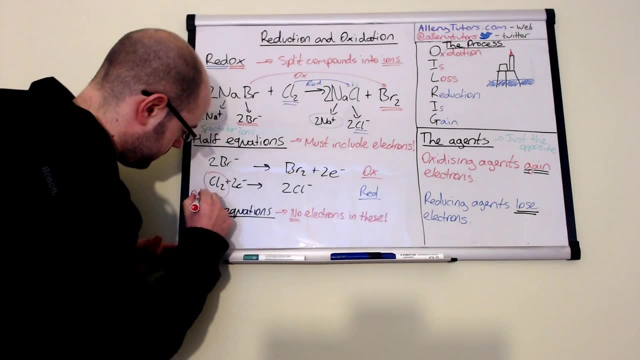 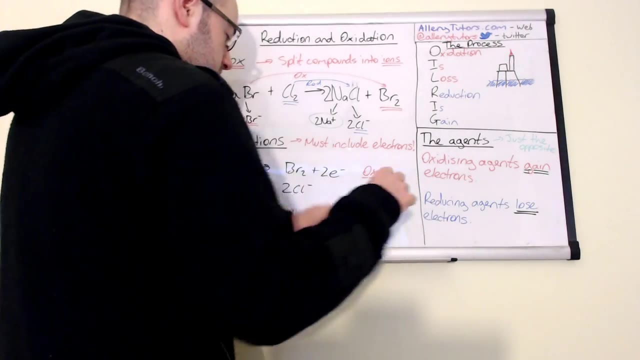 gaining electrons going from left to right. So this one is our oxidizing agent. So I'll just circle that. This is our oxidizing agent, Because you can see, the chlorine is obviously gaining electrons And our Br- is losing electrons, So this is our reducing agent. 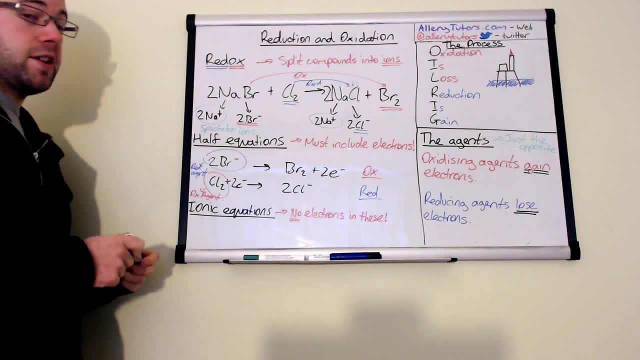 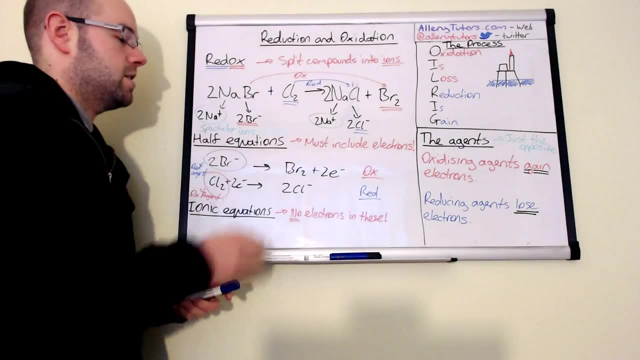 There you go. Okay, So we've identified our oxidizing and reducing agents in this reaction as well. And it'll be the opposite way if you were going back to front, But this reaction is going from left to right. So these are our oxidizing and reducing agents. Okay, So once.